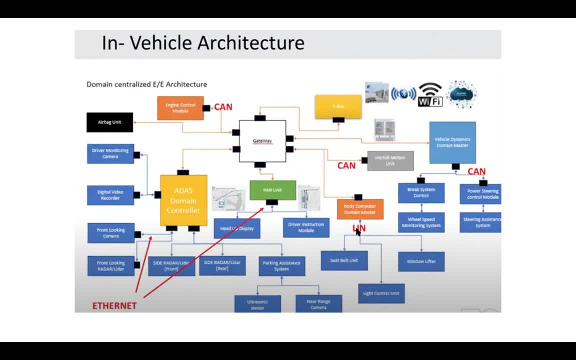 control, for that matter. So there we set a specific speed at which we want our vehicle to move And also the distance, like between the distance that needs to be maintained between the ego vehicle and the vehicle ahead. Ego vehicle is our vehicle and the vehicle ahead. 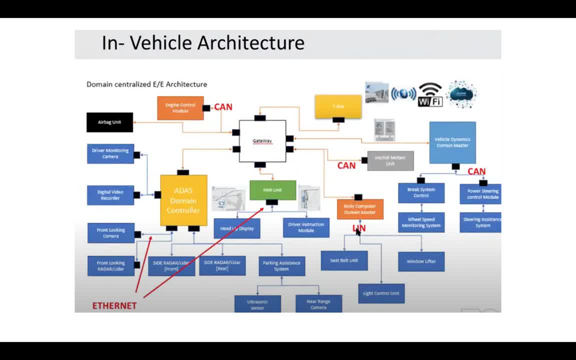 So say, for example, as soon as we have- you know- traffic ahead, then what? what this adaptive cruise control functionality does is that it tries to decelerate it. It's tried to. it tries to brake and slow down. And as soon as the traffic is clear, 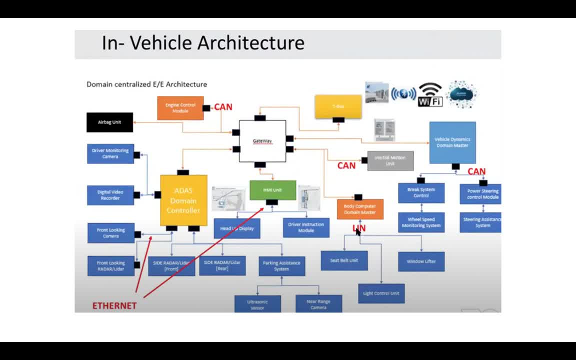 it tries to maintain the same speed that is being set by the user. So for such applications, for such applications, it's very critical and also life threatening as well. So the data needs to be very, very much consistent and very much immediate. 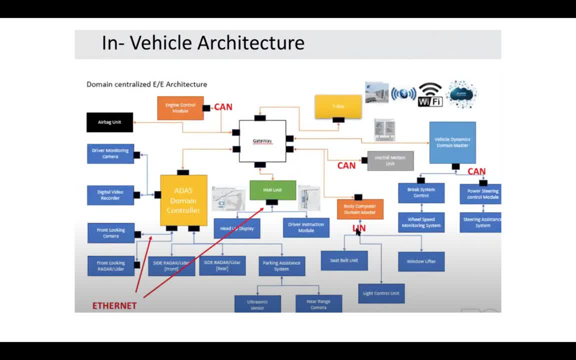 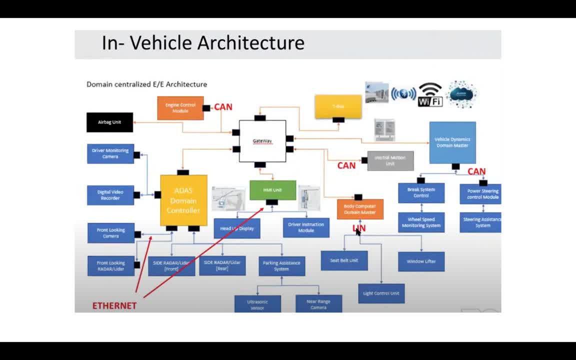 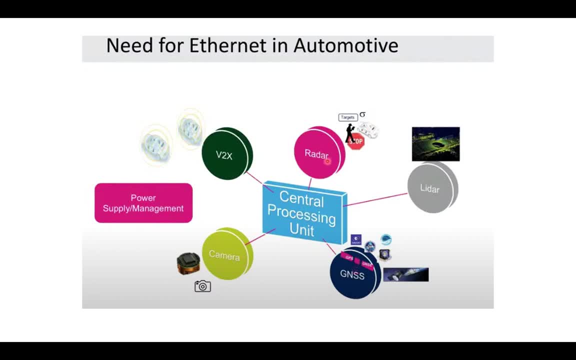 very, very, very important And so it's a really important place. So many people have listened to어�un friends and been that it makes sense to love some of these products. But if you are a car and you are a home car like you're building, 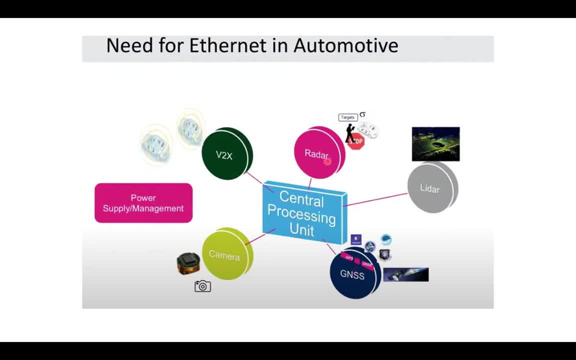 I know many people think that you could be with your car for ruler Washing300.. Well, you can free a few tasks when I uhTalk about the AT&T system, the GNSS 218.. The wavering AT&T system. So, if we're talking about IoT, IoT has a lot- and all the digital devices in the market. 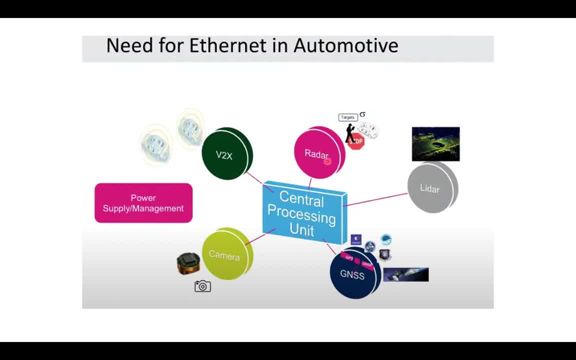 we are talking about using WhatsApp. We use WhatsApp, Uh huh. huge set of applications and huge set of data, and the processing of this should be done at a higher speed and also the transmission and reception should go on at a higher speed. So for these things, in these areas, Ethernet plays a major role, and when it comes to the 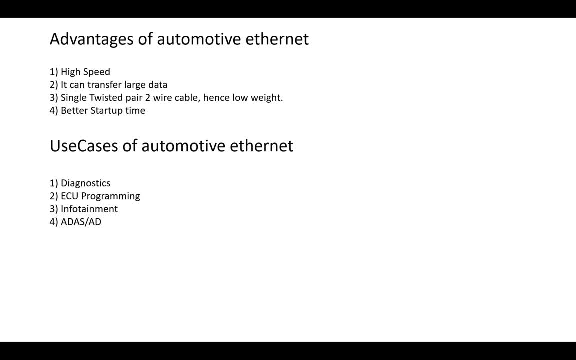 advantages of Ethernet. when it comes to the advantages of Ethernet, as I already mentioned, that is the high speed and also it can transfer large data like speed, like 100 Mbps, 10 Mbps, like we have a flexible speeds there, 2.55, 10 Mbps is also there and also now the 25 Mbps. 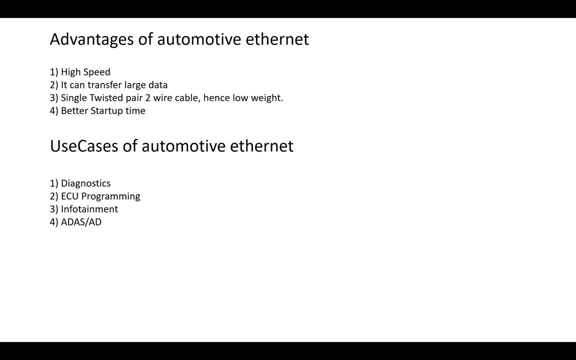 is being about to be standardized and also it can transfer large data like in one frame, like around 46 to 1500 bytes per second. It can be transferred and also single twisted pair 2 wire cable, so the low weight like, because we cannot put huge cables like, say, for example, if we take the consumer automotive, like there. 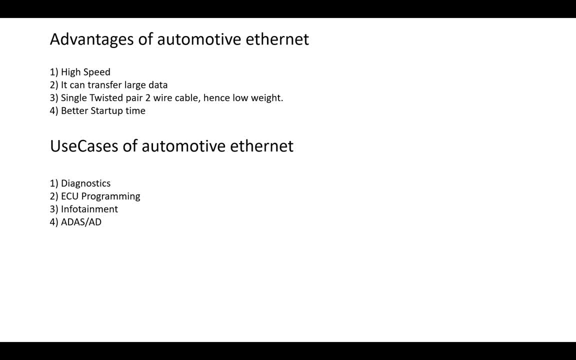 they have 4 or 8 wire, like 4 wire twisted pair cable so that so much of wire cannot be put it in, put in the- you know our automotive or vehicles. so, but by this you know single twisted pair 2 wire cable. the weight is also less and also the better start up time that 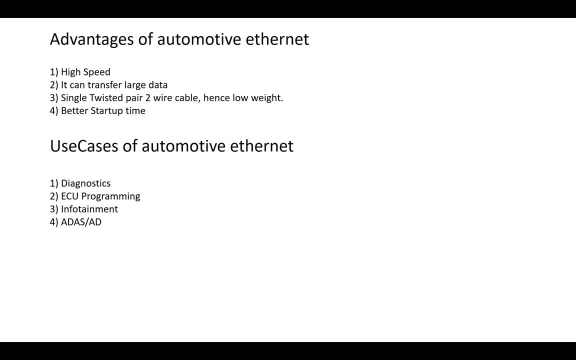 is also one of the advantage. yes, of course, we will discuss these points one by one. and also let's speaking about the use cases, the use cases that we have, the automotive use cases, like for mainly for the diagnostics. so yeah, the ECU programming and infotainment. 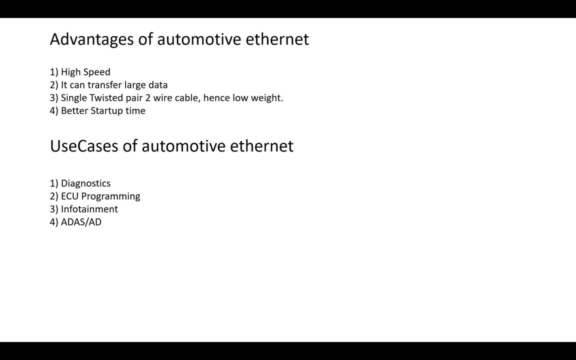 infotainment is not just the navigation and audio, But there are also other applications, like we can transfer a video show, a video image, like a DVD image, the rear view camera, the surround view, etc. So we can also stream audio inside the car into the car from outside. yeah, 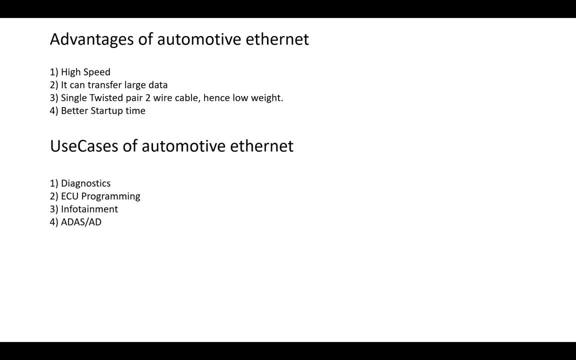 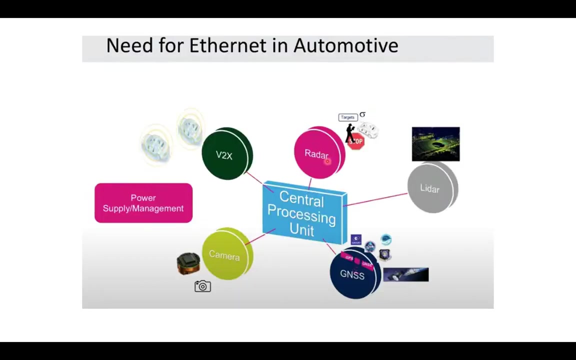 So these are some of the you know applications or use cases from infotainment, and also the advanced driver assistance system or autonomous driving, like the data coming in or going like from. you know the radar leaders, camera image sensors, etc. So now now considering the automotive Ethernet. automotive Ethernet, the physical layer concerning 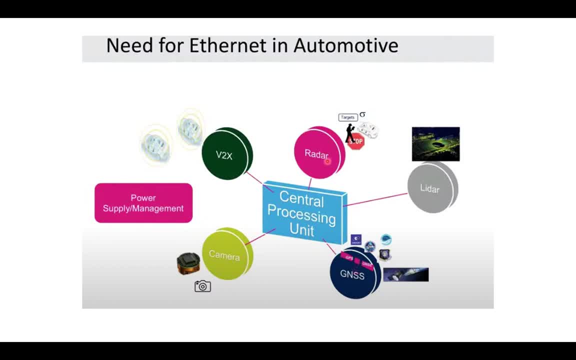 the physical layer. so what is this physical layer? physical layer, make sure that you know it transmits the data over your medium. that could be a cable, fiber optics or could be one radio waves. On Ethernet, we basically have different requirements in the car, So it's not the same as your consumer Ethernet. it's a little, it is bit different from that. 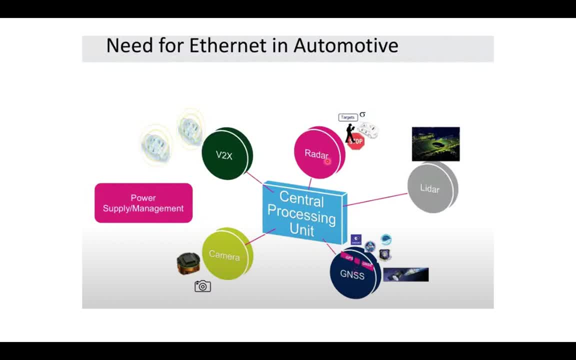 that we have in the enterprise Ethernet, yeah, or you have, you know, or the one that we have in our home, for instance for the Ethernet. So, for example, if we, you know, start a gigabit Ethernet link at our home, It can take up to around, you know, three to one to three seconds until the link is ready. 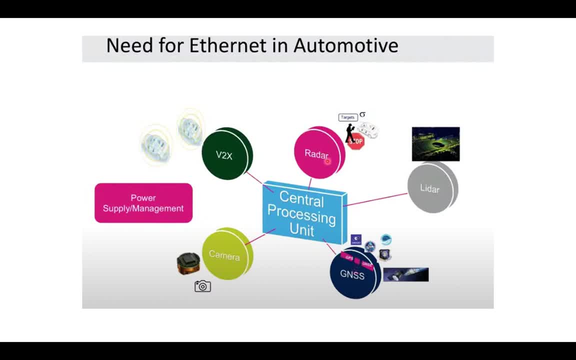 to be, you know, ready for transmission of data. So this is not good in our automotive case or in our car. So if you have something inside the car, you want that application to be available faster, like, just as an example, if you take like five seconds or three seconds to open the door. 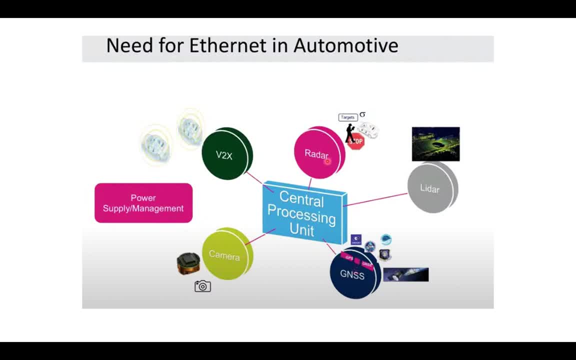 or start the engine. So this is practically not possible. So we want to make you know, make it faster, and a typical use case says that around below 200 milliseconds as a startup time, That could be a good one. So if we also look at the connectors, for instance in the enterprise Ethernet, you know, we typically 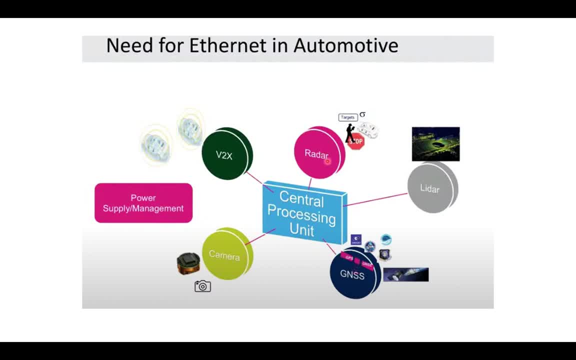 use RJ45 connector which has around eight pins, So you know four twisted pins, So you can see that there is a pair of wires in that. So those have some problems with respect to automotive, like, say, we have our vehicle moving and the pressure or mechanical movement would be an issue, and also connector should be stable. 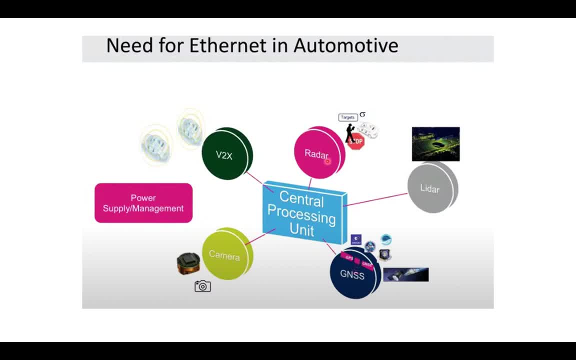 The connectors that we use in our automotive Ethernet should be stable. It should be able to withstand the pressure, mechanical movement, vibrations, EMI, EMC, etc. And also humidity could also be a problem, like if the water gets in, So there should be a change in the connectors. 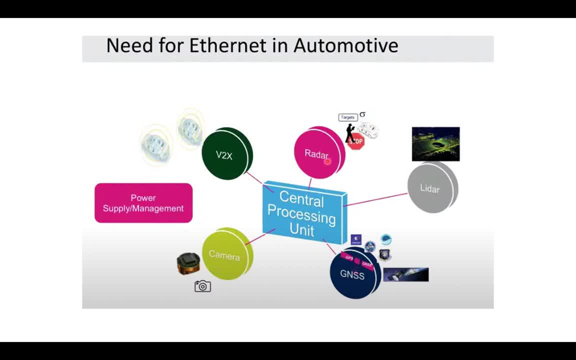 Okay, So these are the connectors that we use in the enterprise Ethernet to the automotive Ethernet. So that's why, you know, no single twisted pair cable is being used, which is, you know, electromagnetic wave compatible as well, Compatible as well. Yeah, Now, considering all these things, considering all these things like the startup time, the 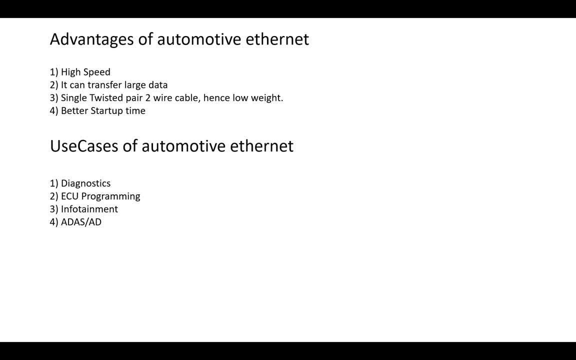 EMI, EMC, the weight, the connectors. If we look at these, you know use cases that we just discussed. Yeah, The software update in the car, the ECU programming, whatever I mentioned, we don't know. we don't have that hard requirements in the car like when it comes to ECU programming, because car 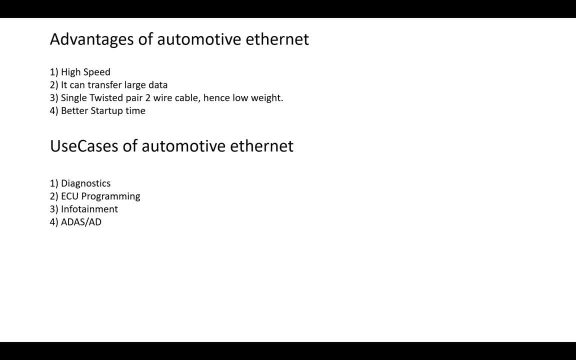 is not moving standing. It is standing still in the shop or in the service center. So here we could use the regular standard like 100 base TX. So it's the same that we use on our notebook or on our desktop. So no much change with respect to. 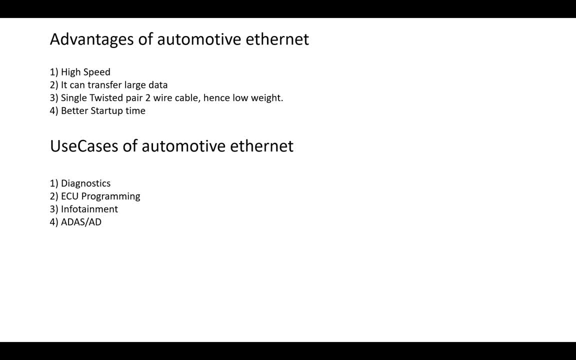 The enterprise Ethernet or no change required here. But if we consider that enormous driving or advanced driver assistance system, here the technology has to work like when the when the car is moving, yes, when the car is moving. So here we have to fulfill all the requirements that we just discussed, like the startup time. 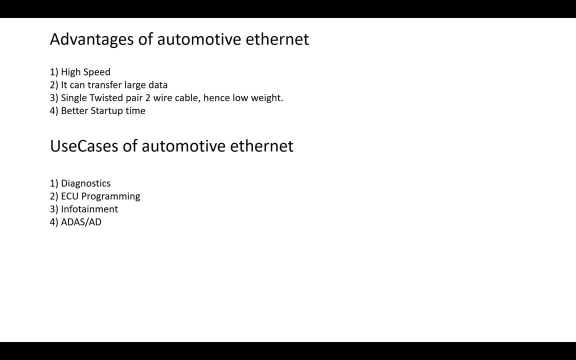 of the, you know, Ethernet link or EMI, EMC, or the weight, the connector, connectors and so on. So what happens here is that the special physical layer transverse has to be connected, So the physical layer has to be created. So it's all. now, in the current market we already have 100 base, 10 base, 1000 base, 2.5 or 5 or 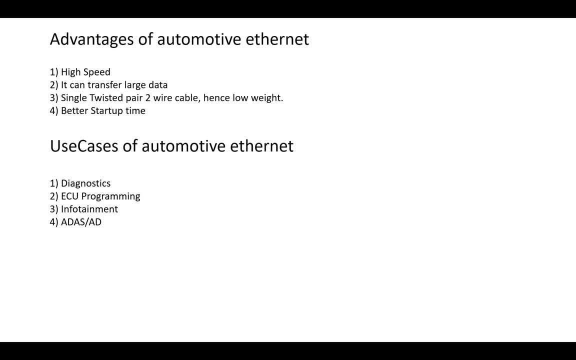 10 gigabits already available, So which can be made use in our applications. Yeah, And also one thing is that we don't use automotive Ethernet Just for physical layer, the terminology automotive Ethernet just for not just for our physical layer but everything on top of that, like if you run on top of that at the top of the Mac. 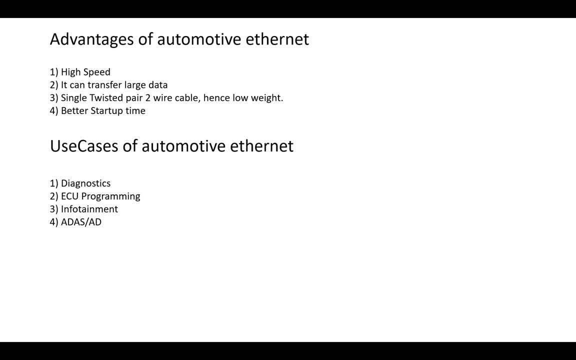 layer, you know Mac layer with VLAN, or you run your precision timing protocol for time synchronization. or if you run the QS mechanisms like shaping, prioritization, policing, the time sensitive networking. But Yeah, Also you can run the TCP IP stack on top of that or UDP IP stack on top of that. 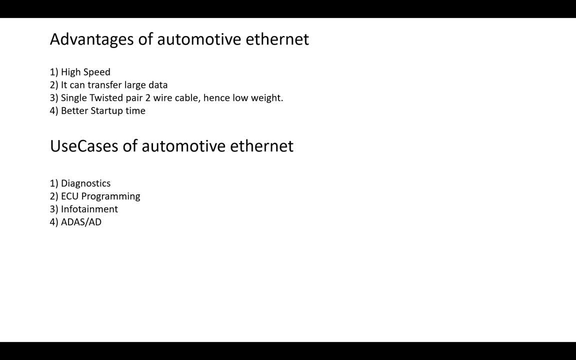 Also you can run the audio video bridging on top of that, like AVB, as well as the, the some IP, Yeah, The middleware for control messages, Of course, the diagnostic or Internet protocol to do the flash update or ECU programming. So this was all about regarding the you know introduction. 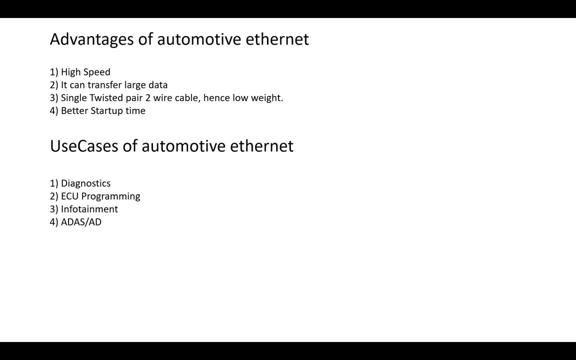 Or you know basics of automotive Ethernet. Thanks for watching the video. If you like this video, please give it a thumbs up. 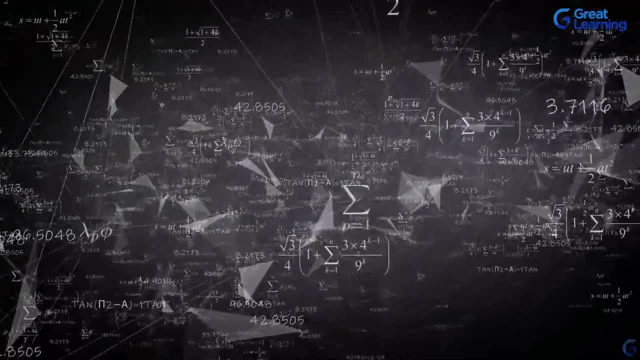 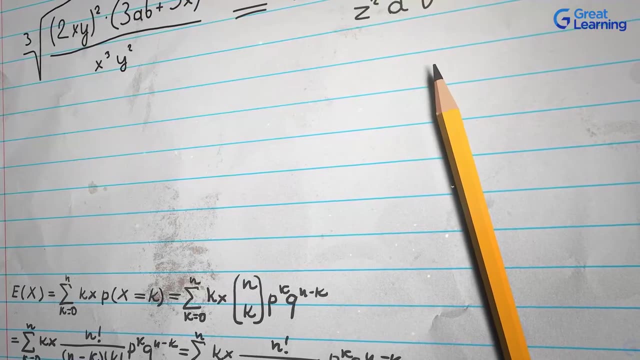 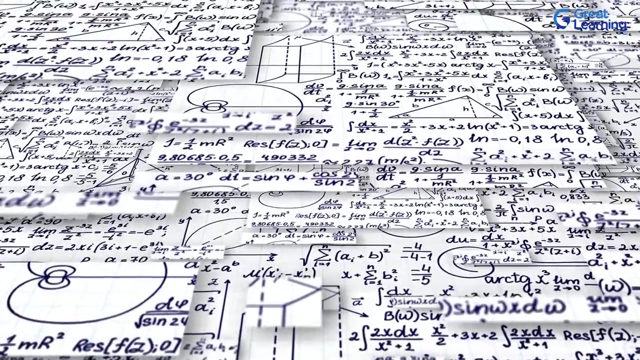 Discrete mathematics is the mathematical concept concerned with concepts that can only have independent, isolated values. As a result, the term discrete mathematics is used in opposition to constant mathematics, which is the field of mathematics concerned with objects that can fluctuate gradually. It helps us in identifying and further analyze various components of computer. 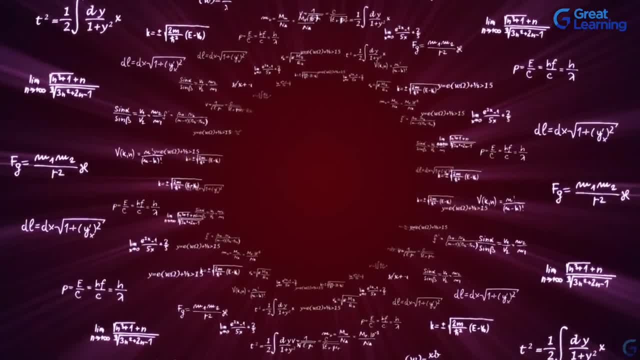 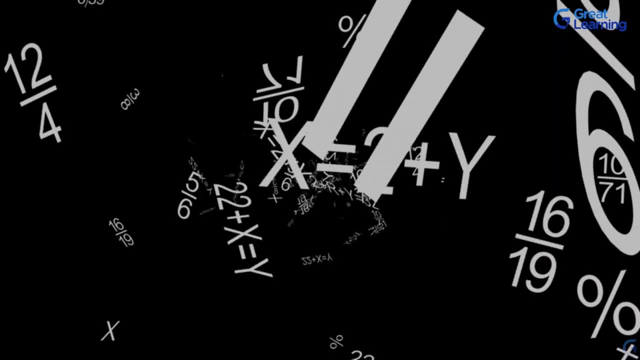 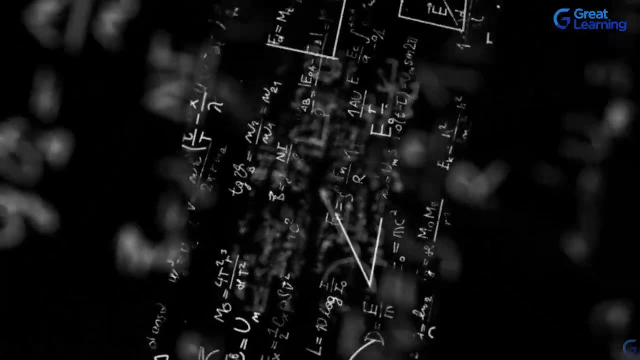 science that actually practically utilize discrete value in their execution. Through this video, we will be understanding some basic concepts in discrete mathematics, namely set relation and function theory, and understand exactly how they interact with one another. We will also be looking into concepts like counting principle and propositional logic. 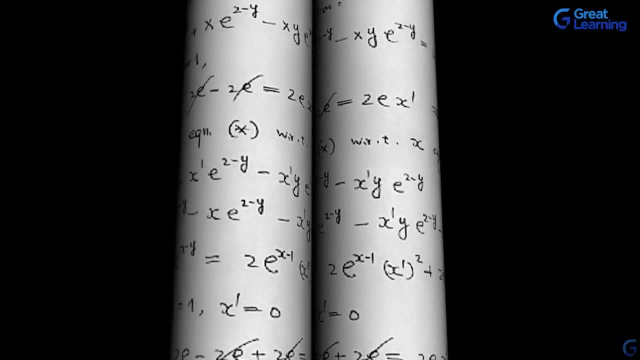 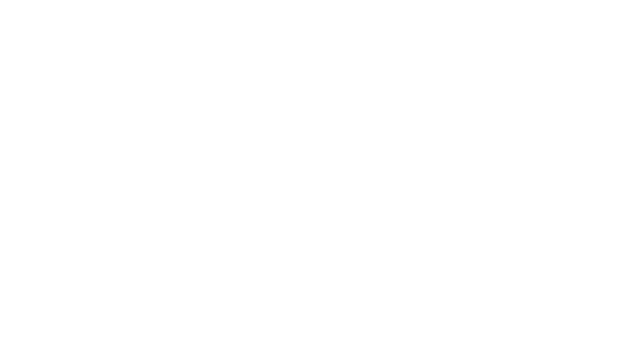 that consider the set and relation theory as its base, and a whole lot more. So put on your thinking hats and let's get started with this session on basics of discrete mathematics. If you haven't subscribed to our channel yet, I want to request you to hit the subscribe button. 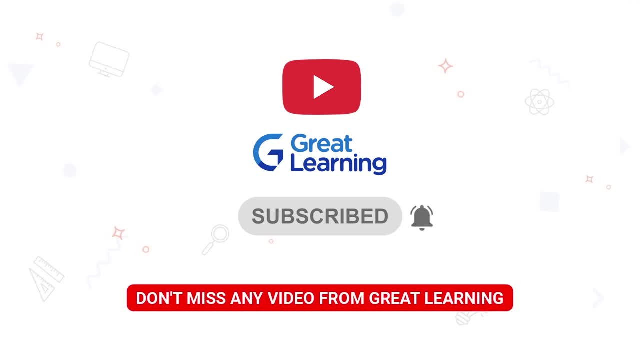 and turn on the notification bell so that you don't miss out on any new update or video releases from Great Learning. If you enjoy this video, show us some love and like this video. Knowledge increases by sharing, so make sure you share this video with your friends and colleagues. 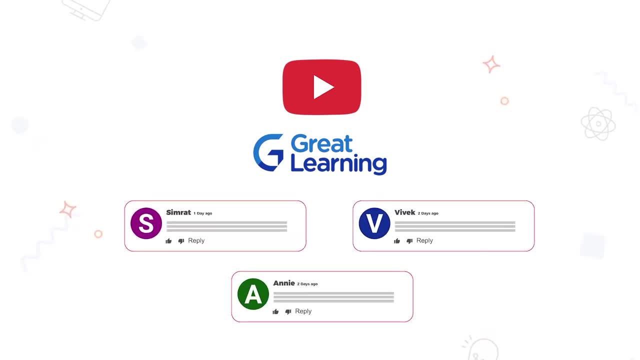 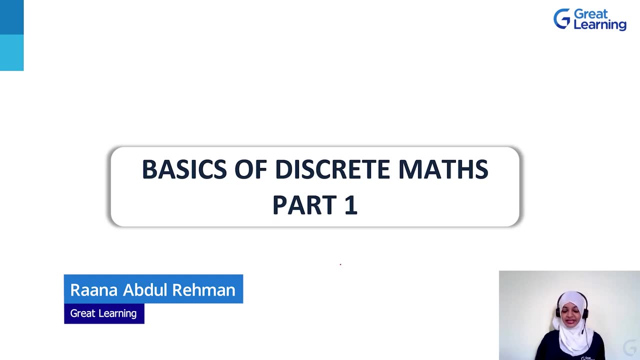 Make sure to comment on the video for any query or suggestions, and I will respond to your comments. Hello everyone, Welcome to a new course known as Basics of Discrete Maths. In this particular course, we'll be understanding what discrete maths is and how it helps us. Often, students learning this course have a question.